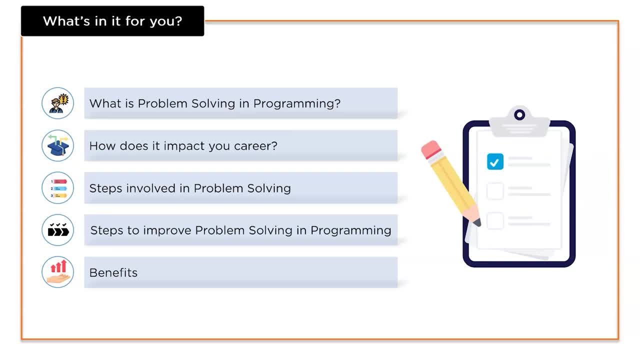 discussing benefits of problem solving and programming. However, before we begin, make sure that you have subscribed to our YouTube channel and don't forget to hit that bell icon so you never miss an update from Simply Learn. Let's start with what is problem solving and 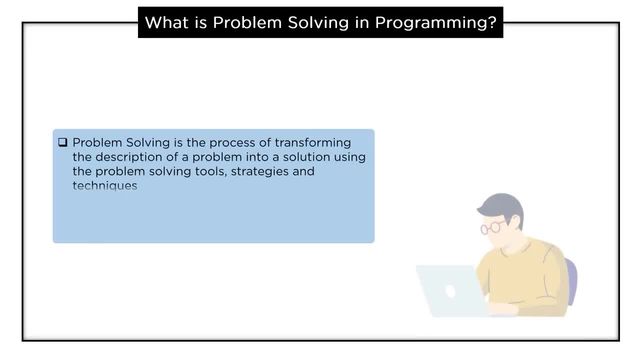 programming. Computers are used to solve various problems in day-to-day life. Problem solving is an essential skill that helps to solve problems. in programming, Problem solving is the process of transforming the description of a problem into a solution, using the problem solving tools, strategies and techniques. Computers act as helpers to solve. 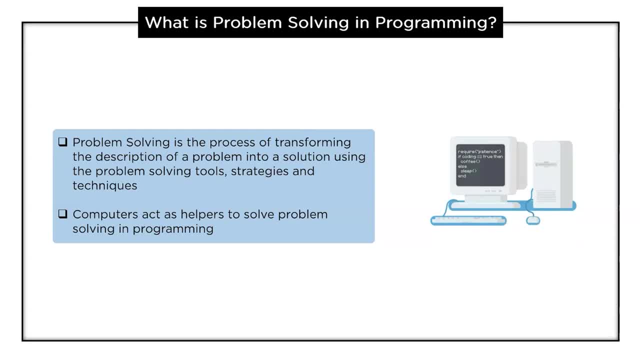 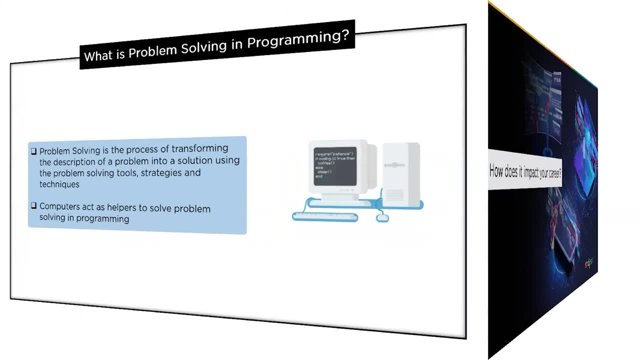 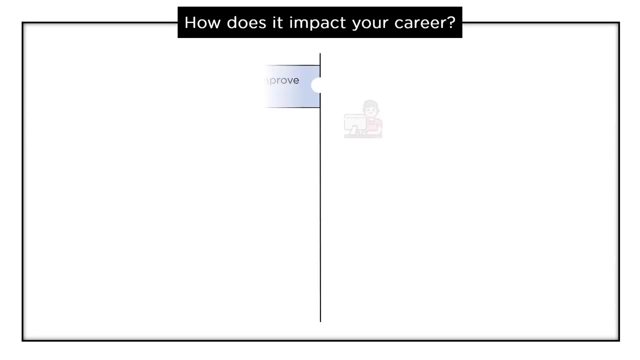 problem solving in programming. This involves designing, identifying and implementing problems using specific steps to develop a computer. Now let's have a look at how problem solving has an impact on a career. Many companies look for candidates with excellent problem solving skills. For example, a computer can be used to solve problems in programming. A computer can. 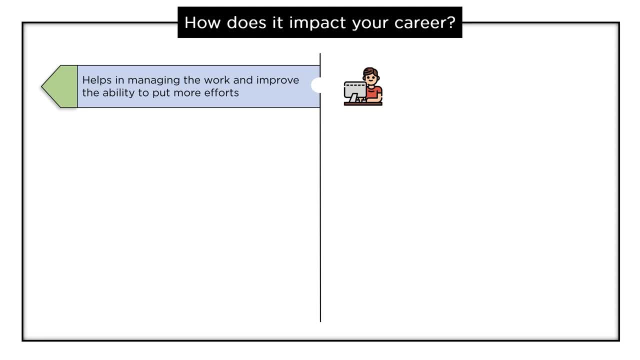 help people manage the work and make candidates put more effort into the work, which results in finding solutions for complex problems in an unexpected situation. These skills also help to identify quick solutions when they arise and are identified and shown possible results for complex problems. Problem solving skills also improve thinking and analytical skills, which 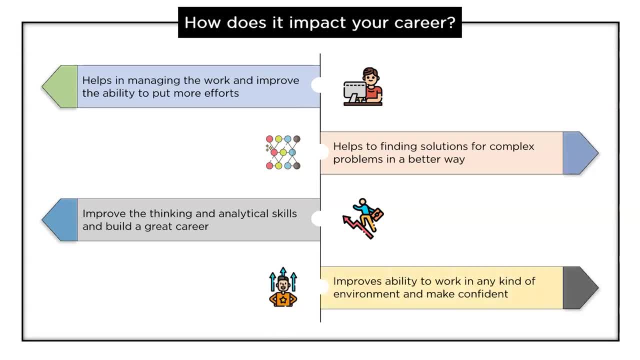 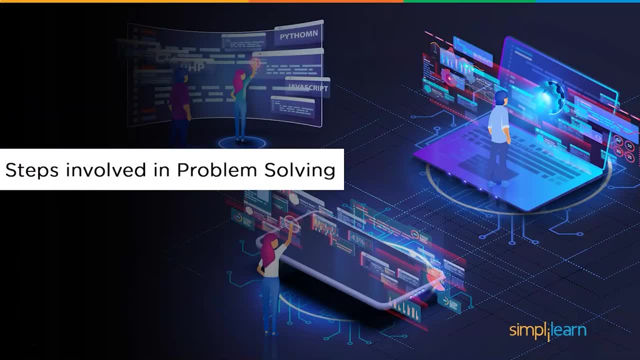 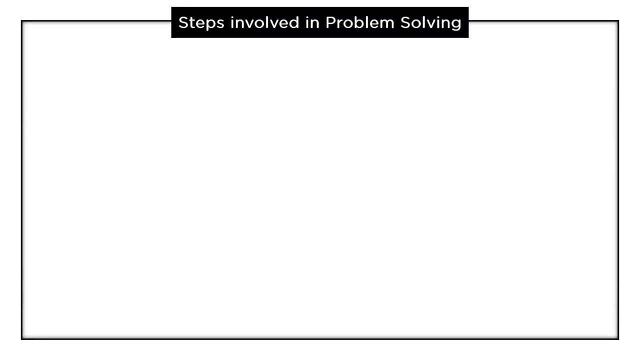 make them much more successful. Problem solving skills also help build confidence in their career and work in any kind of environment. Now let's start with learning the steps involved in problem solving. in programming, Before being ready to solve a problem, there are some steps, and 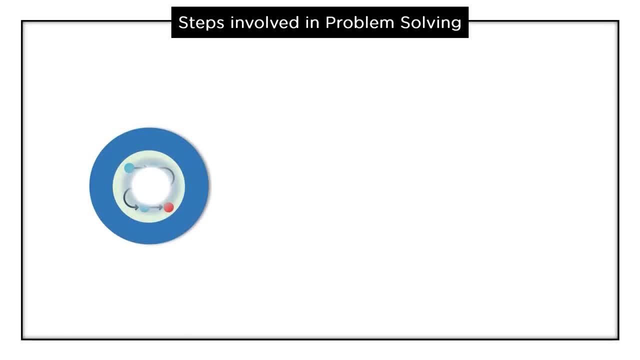 procedures to be followed to find the solution. Now let's have a look at them. So these are basically divided into four categories. The first one is analyzing the problem. Next is developing an algorithm, Followed by that we have coding and then we have testing. 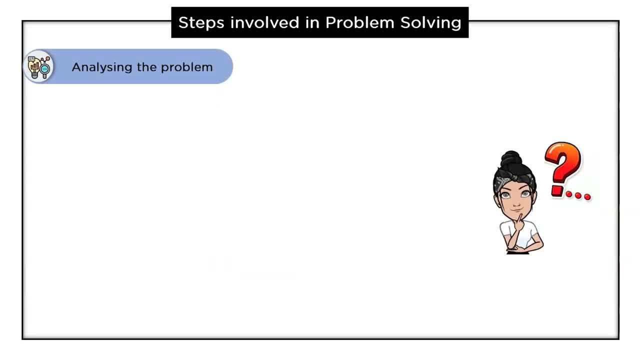 and debugging. Let's walk through them in a deeper and more detailed way. The first one is analyzing the problem. Every problem has a perfect solution. Before we are ready to solve a problem, we must look over the question and understand it. By analyzing it, we can figure out the outputs and 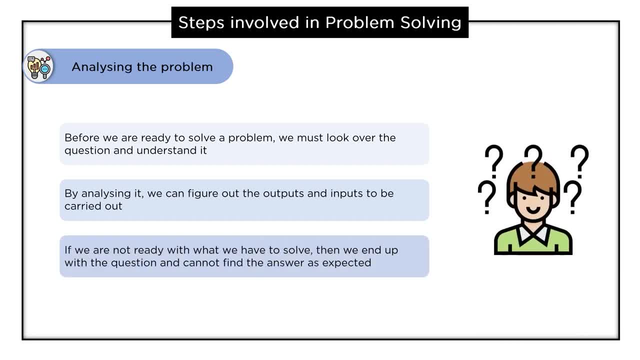 inputs to be carried out before solving. If we are not ready with what we have to solve, then we end up with a question and cannot find an answer as expected. And if you know what you're solving, then this would help you to find a 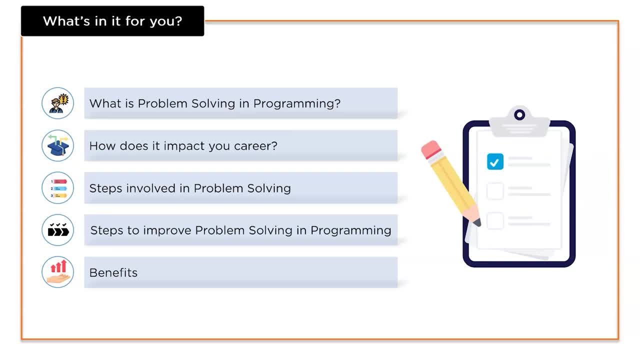 discussing benefits of problem solving and programming. However, before we begin, make sure that you have subscribed to our YouTube channel and don't forget to hit that bell icon so you never miss an update from Simply Learn. Let's start with what is problem solving and 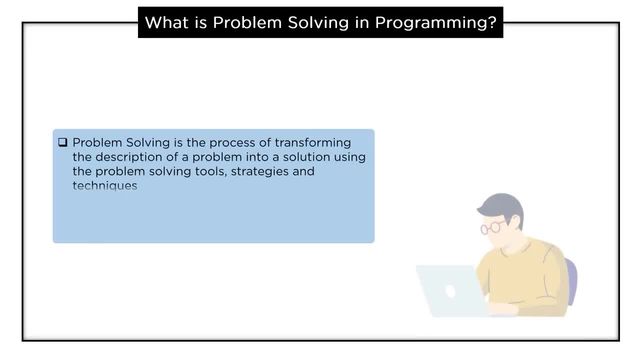 programming. Computers are used to solve various problems in day-to-day life. Problem solving is an essential skill that helps to solve problems. in programming, Problem solving is the process of transforming the description of a problem into a solution, using the problem solving tools, strategies and techniques. Computers act as helpers to solve. 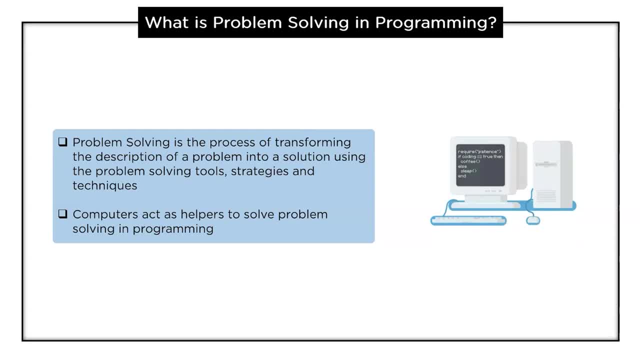 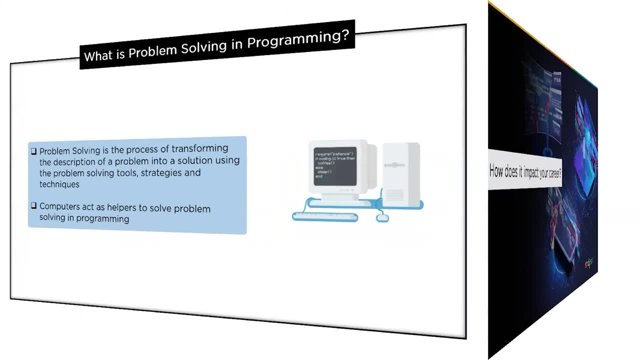 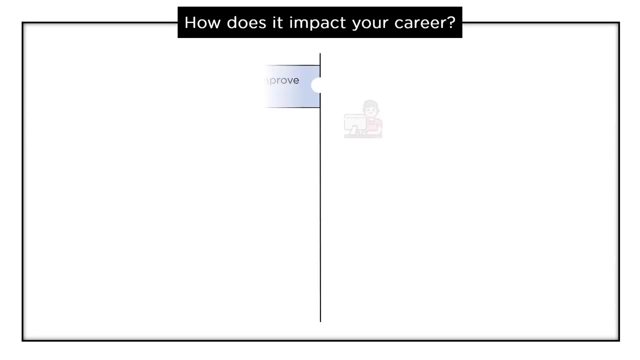 problem solving in programming. This involves designing, identifying and implementing problems using specific steps to develop a computer. Now let's have a look at how problem solving has an impact on a career. Many companies look for candidates with excellent problem solving skills. 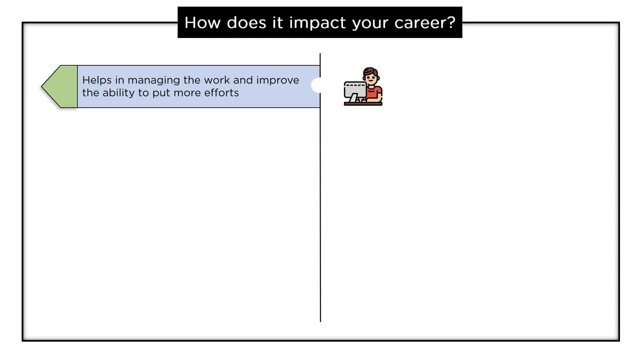 These skills help people manage the work and make candidates put more effort into the work, which results in finding solutions for complex problems in an unexpected situation. These skills also help to identify quick solutions when they arise and are identified and shown possible results for complex problems. Problem solving skills also improve thinking and analytical. 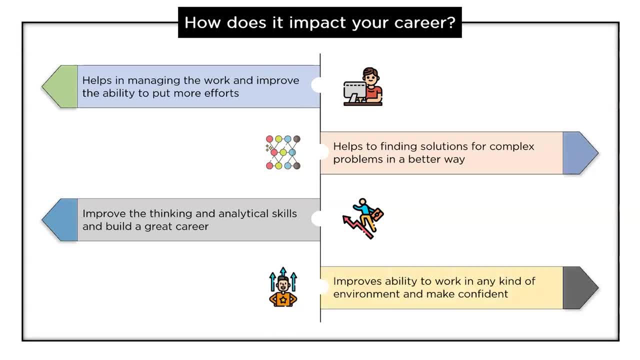 skills which make them much more successful. Problem solving skills also help build confidence in their career and make them more successful. Problem solving skills also help build confidence in their career and make them more successful. Problem solving skills which help build confidence in their career or. 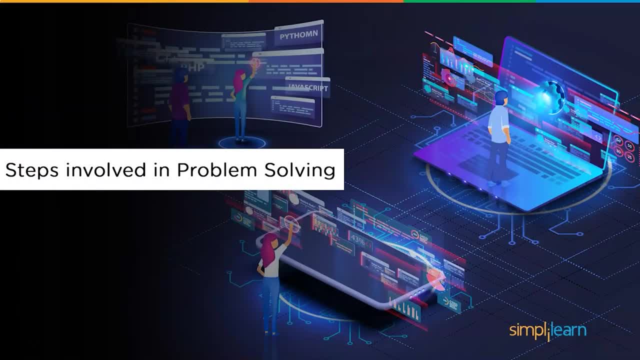 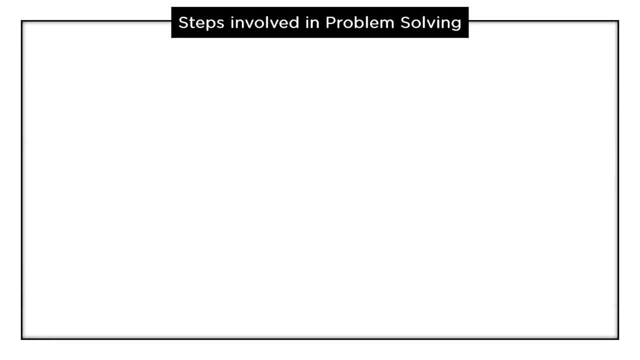 develop confidence in their growth can create access to 20% more money and save around modng $10.. Now let's start with learning the steps involved in problem solving in programming. Before being ready to solve the problem, there are some steps andœ procedures to be followed. 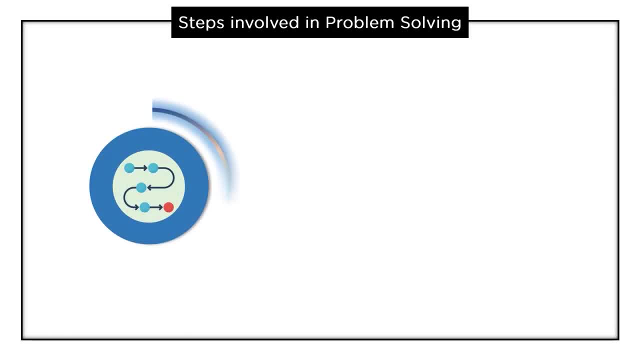 to find the solution. Now let's have a look at them. So these are basically divided into four categories. The first one is analyzing the problem. Next is Developing an algorithm, Followed by That we have Coding, And then we have Testing. 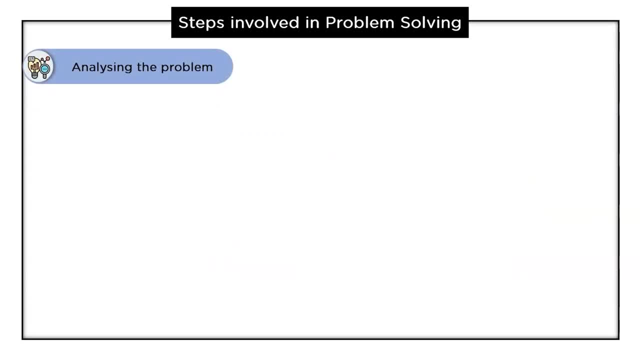 testing and debugging. Let's walk through them in a deeper and more detailed way. The first one is analyzing the problem. Every problem has a perfect solution. Before we are ready to solve a problem, we must look over the question and understand it. 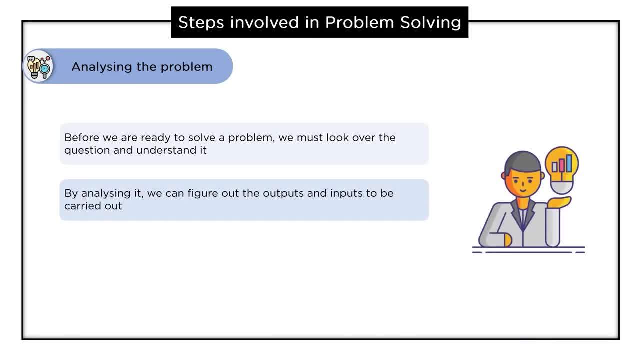 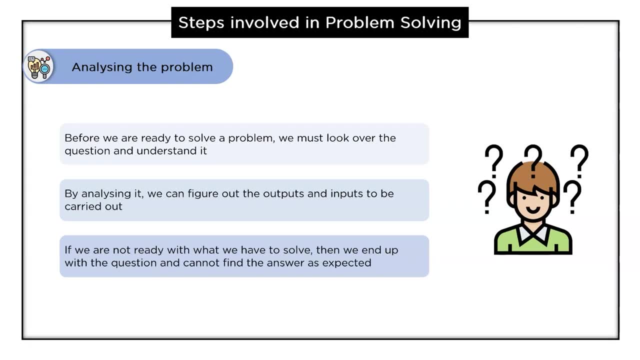 By analyzing it, we can figure out the outputs and inputs to be carried out before solving. If we are not ready with what we have to solve, then we end up with a question and cannot find an answer as expected. And if you know what you are solving, 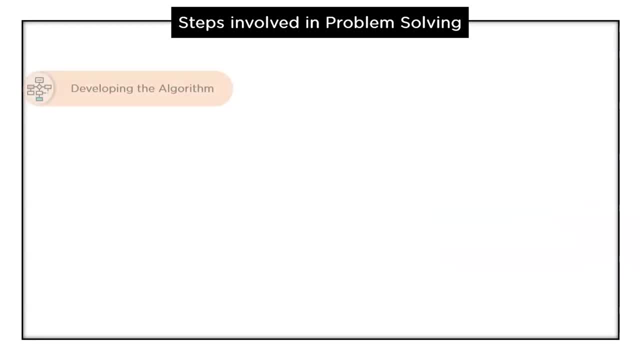 then this would help you to find a solution very easily. The next step is developing the algorithm Before you are ready to solve a problem. it is required to decide a solution before writing the program. The representation of the solution in natural language is called as an algorithm. 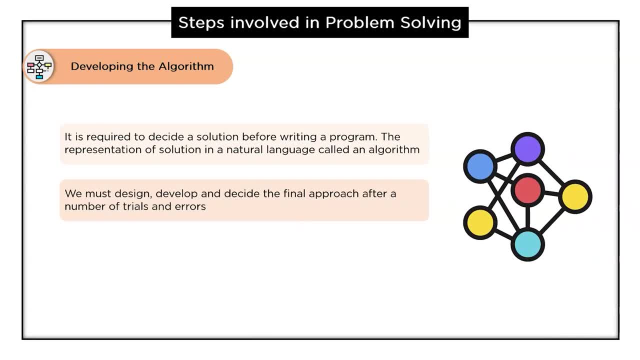 We must design, develop and decide the final approach after several trials and errors, before actually writing the final code on an algorithm. before we write the code: Developing an algorithm is a process that requires a lot of effort and a lot of effort. Developing a solution is a process that requires a lot of effort and a lot of effort. before we write the program. 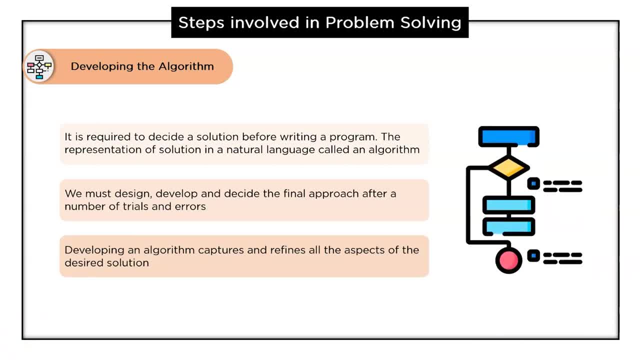 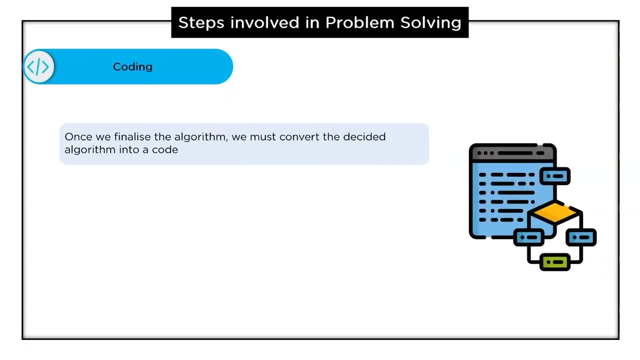 algorithm captures and refines all the aspects of the desired solution and can solve the problems very easily. And the next step in the list is coding. Once we finalize the algorithm, we must convert the decided algorithm into code. Once we are done with the algorithm, we have to code or 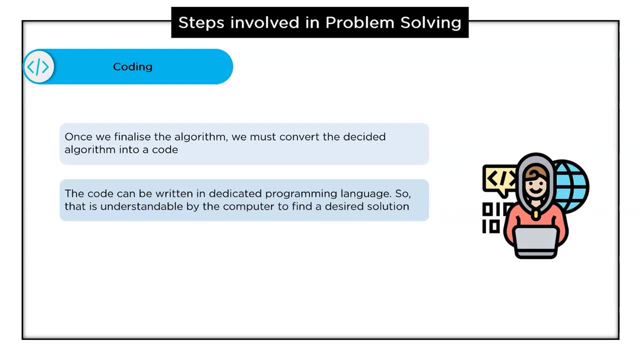 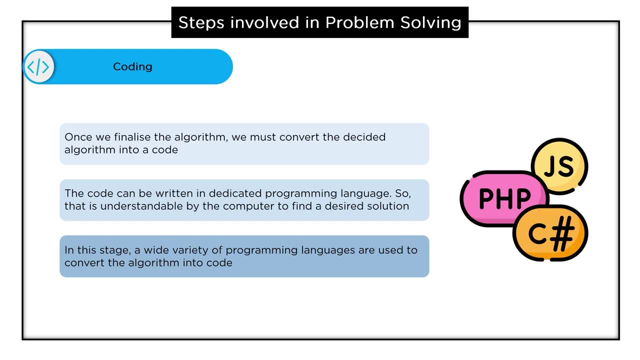 program using a dedicated programming language that the computer understands to find the desired solution. In this step, a wide variety of programming languages are used to convert the algorithm into code. Now let's have a look at the final step in the list, that is, testing and. 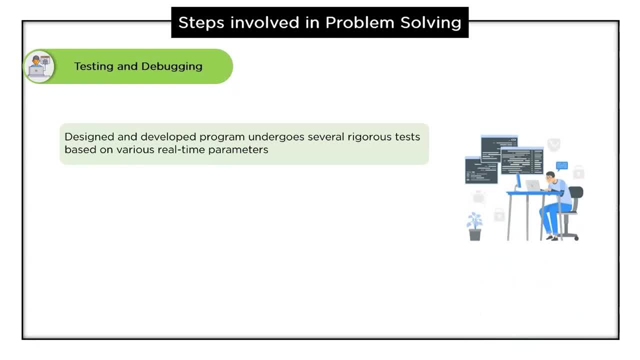 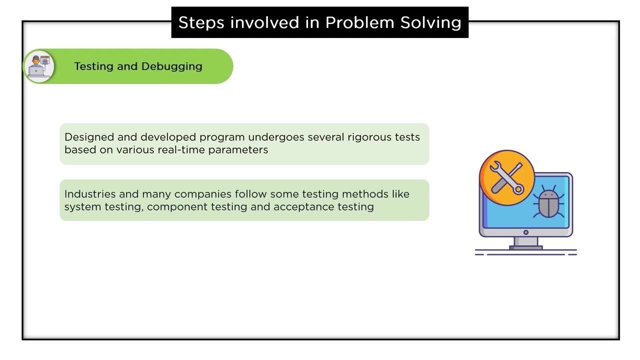 debugging. The designed and developed program undergoes several rigorous tests based on various real-life parameters and the program undergoes various levels of simulations. Industries and many companies follow some testing methods like system testing, component testing and acceptance testing. It should generate all expected outputs to all the possible inputs. The program 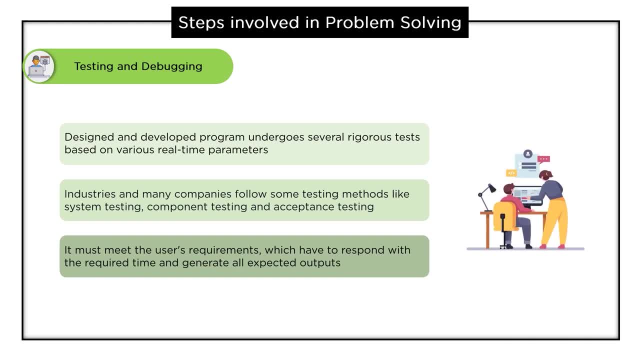 should also undergo bug fixing and all possible exception handling. If it fails to show possible results, it should be checked for logical errors. These are the four steps involved in problem solving and programming. Now let's have a look at the steps to improve problem solving and. 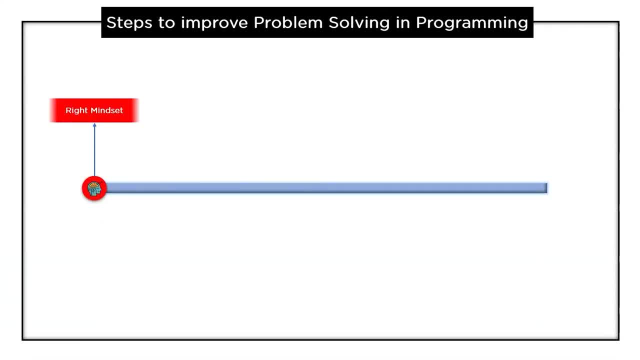 programming. So following are the steps to improve the problem solving and programming. The first one is the right mindset. Followed by that, we have making right decisions. Next, we have keeping ideas on the right mind set. Next, we have keeping ideas on the right mind set. Next, we have keeping 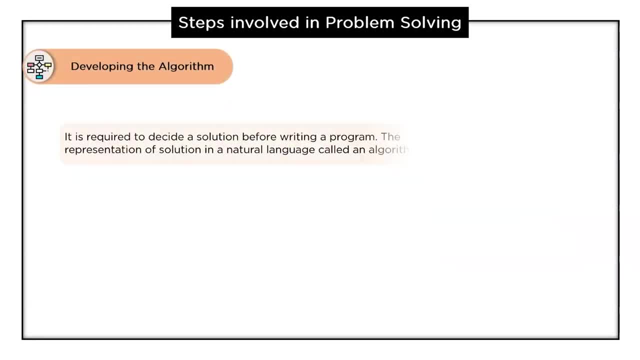 solution very easily. The next step is developing the algorithm. Before you're ready to solve a problem, it is required to decide a solution before writing the program. The representation of the solution in natural language is called as an algorithm. We must design, develop and decide. 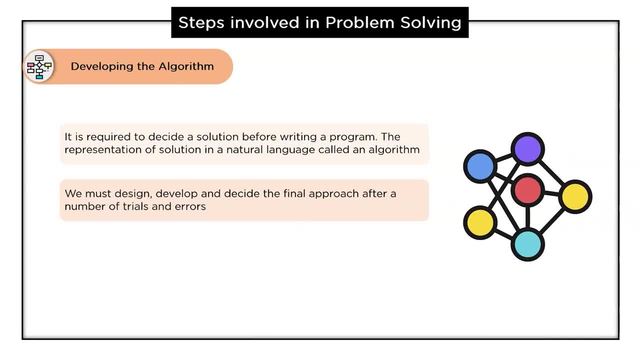 the final approach after several trials and errors, before actually writing the final code on an algorithm. before we write the code, Developing an algorithm captures and refines all the aspects of the desired solution and can solve the problem. The next step is developing the algorithm Before. 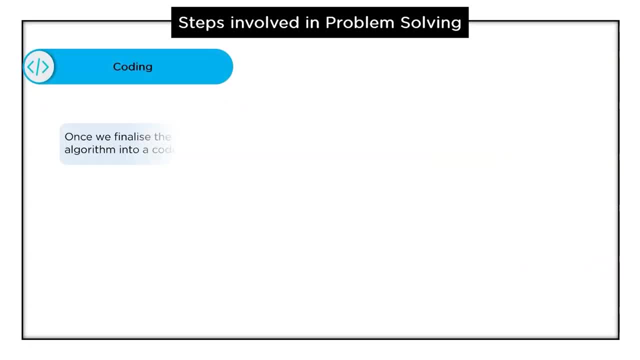 we are ready to solve a problem. we must decide a solution before actually writing the problem. The problem is easy to solve. The next part is coding. Once we finalize the algorithm, we must convert the decided algorithm into code. Once we are done with, 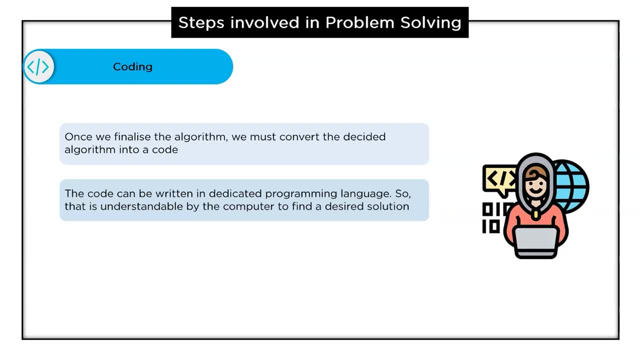 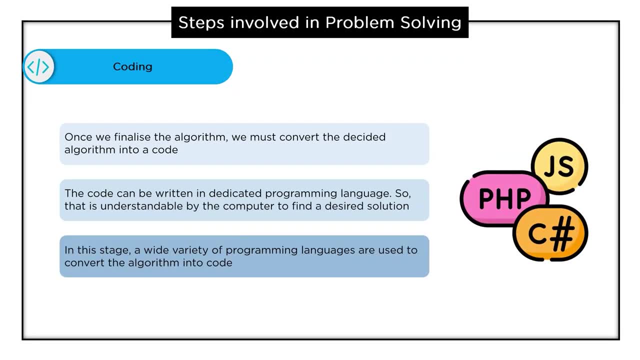 the algorithm. we have to code or program using a dedicated programming language that the computer understands to find the desired solution In this step. a wide variety of programming languages are used to convert the algorithm into code. Now let's have a look at the final step in the list, that is, testing and debugging. 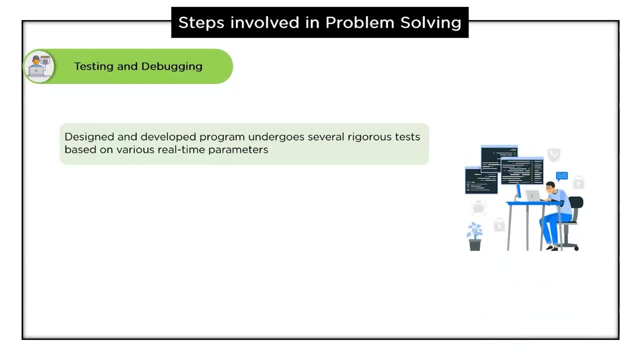 The designed and developed program undergoes several rigorous tests based on various real life parameters, and the program undergoes various levels of simulations. Industries and many companies follow some testing methods like system testing, component testing and acceptance testing. It should generate all expected outputs to all the possible inputs. 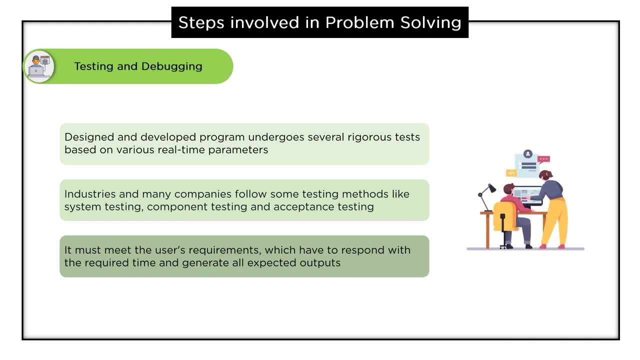 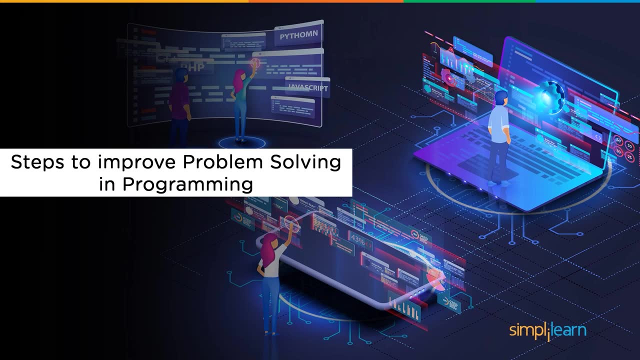 The program should also undergo bug fixing and all possible exception handling. If it fails to show possible results, it should be checked for logical errors. These are the four steps involved in problem solving and programming. Now let's have a look at the steps to improve problem solving and programming. 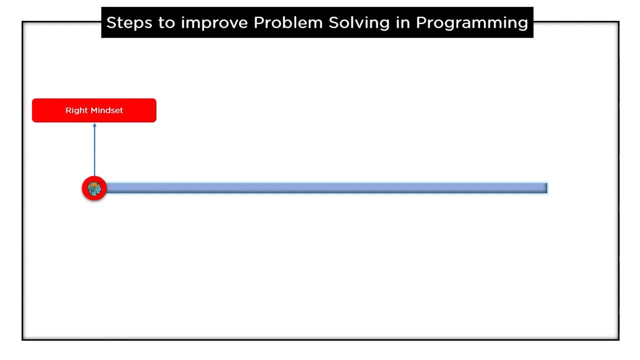 So following are the steps to improve the problem solving and programming. The first one is the right mindset. Followed by that, we have making right decisions. Next, we have keeping ideas on track, Followed by that we have learning from the feedbacks. 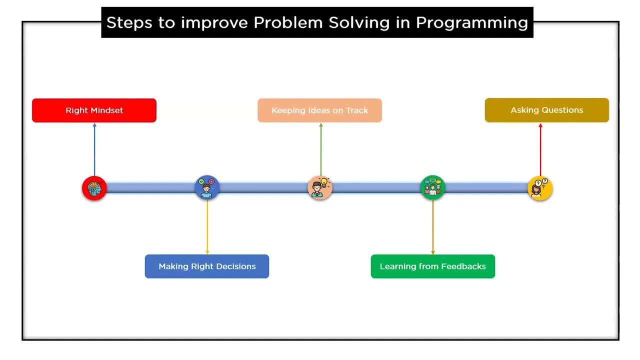 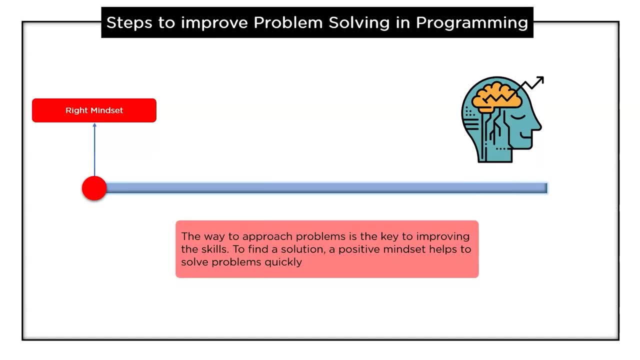 And finally we have asking questions. Let's discuss each one of them in detail. The first one is right mindset. The way to approach problems is the key to improving skills To find a solution. the positive mindset helps to solve problems quickly. If you think something is impossible, then it is very hard to achieve. 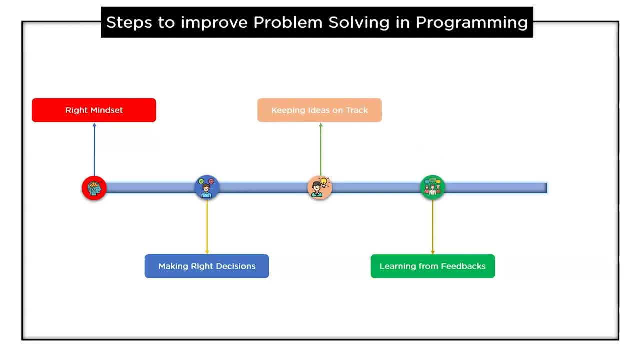 track. Followed by that, we have learning from the feedbacks and finally, we have asking questions. Let's discuss each one of them in detail. The first one is right mindset. The way to approach problems is the key to improving skills To find a solution. the positive mindset helps to solve. 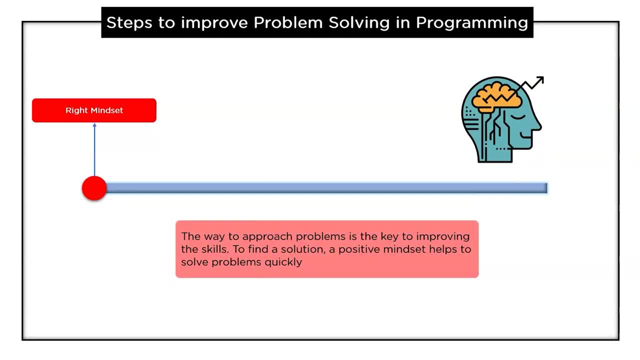 problems quickly. If you think something is impossible, then it is very hard to achieve. Followed by that, we have making right decisions. When we have to solve a problem, we must be clear of the solution. The perfect solution helps to get success in a shorter period. Making the right. 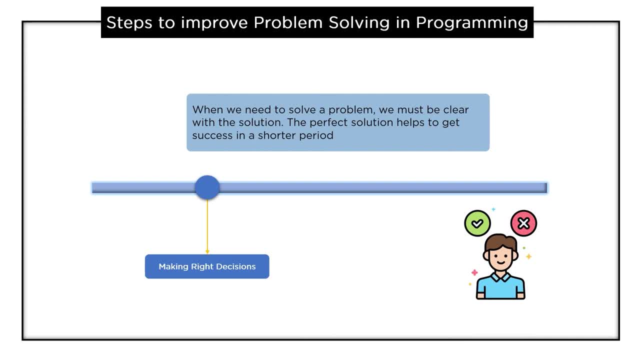 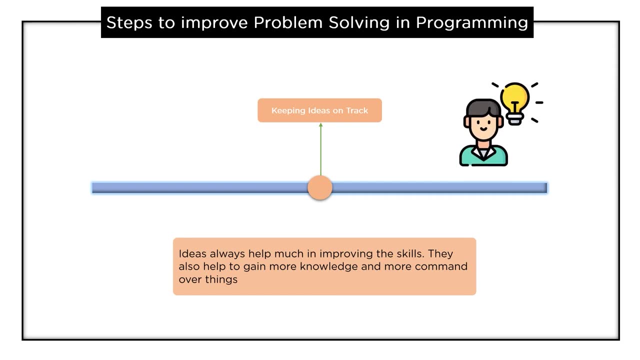 decisions in the right situation helps people find perfect solution quickly and efficiently. These skills also help to get more command over the subject. Followed by that, we have the next step, that is, keeping ideas on track. Ideas always help much in improving the skills. They also help. 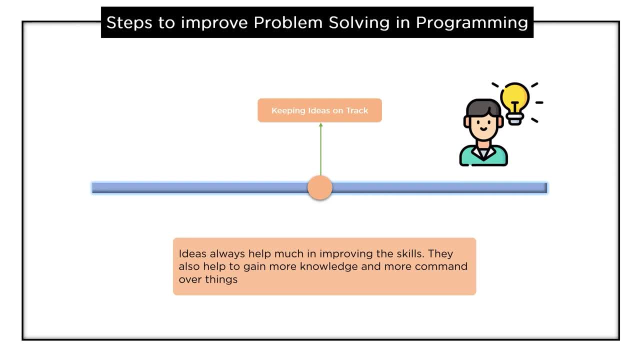 to gain more knowledge and more command over things. In problem solving situations, these ideas help much. We also have learning from feedbacks. A crucial part of learning is the feedback. Mystics help you to gain more knowledge and have much growth When you have a solution for. 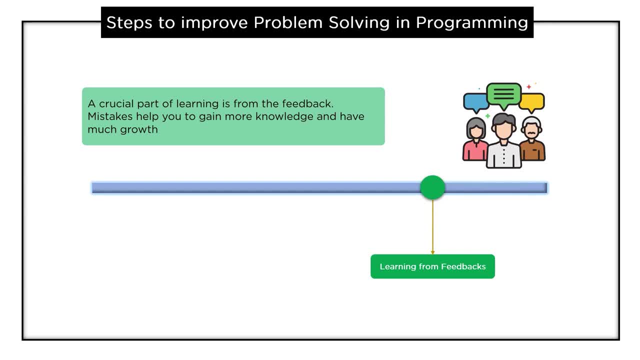 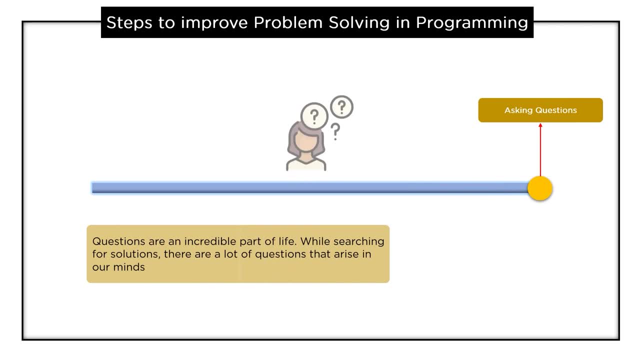 a problem, go for a feedback from experienced or the professionals who are seniors to you. The last one is asking questions. Questions are incredible part of life. While searching for solutions, there are a lot of solutions. They help us develop more knowledge And keep on noting the. 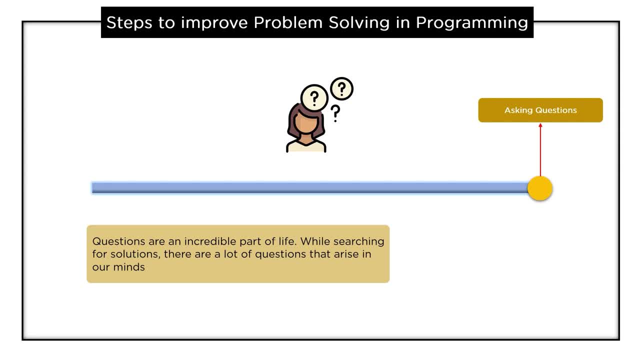 ideas, Give opportunities for the mind and keep on noting the ideas. Next we have learning from are a lot of questions that arise in our minds. Once you know the question correctly, then you can find answers quickly. In coding or programming, we must have a clear idea about the problem. 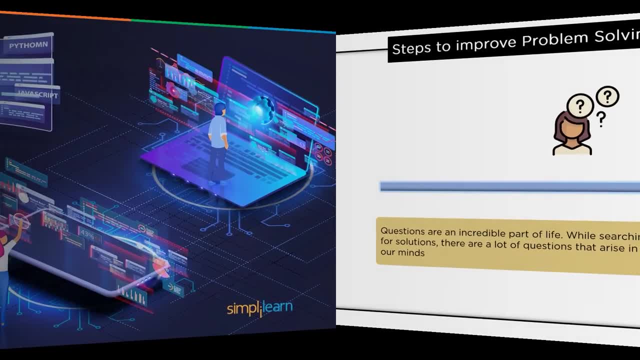 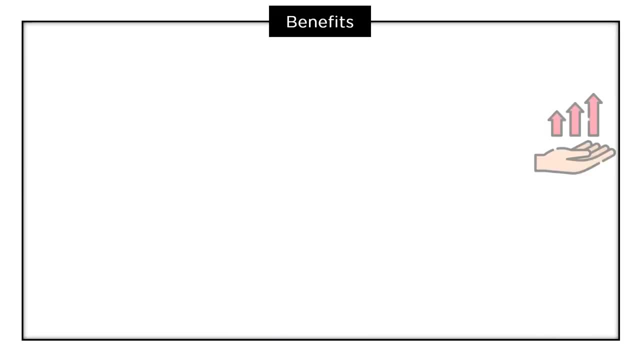 Then you can find the perfect solution for it. So these were some of the important steps to improve problem solving skills in programming. Now let's learn about some important benefits of problem solving in programming. So the first one is: the major benefit of problem solving is to 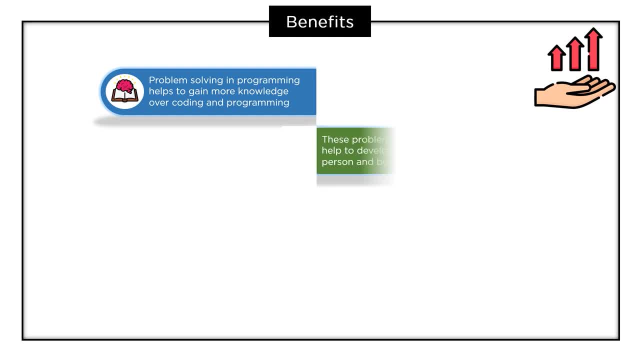 gain more knowledge over coding and programming. These problem-solving techniques and skills also improve the knowledge in a person and build a promising career. These skills play an important role when it comes to jobs. Most of the companies are looking for people with good problem-solving. 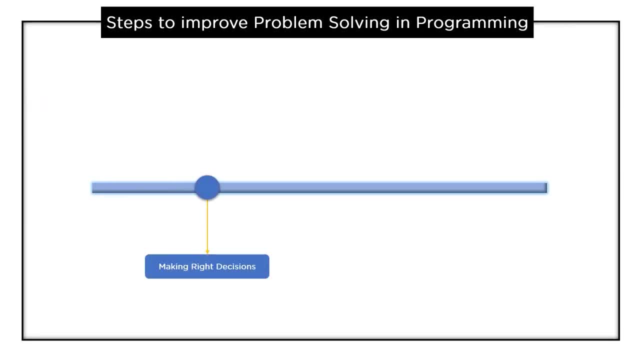 Followed by that, we have making right decisions. When we have to solve a problem, we must be clear with the solution. The perfect solution helps to get success in a shorter period. Making the right decisions in the right situation helps people find perfect solution quickly. 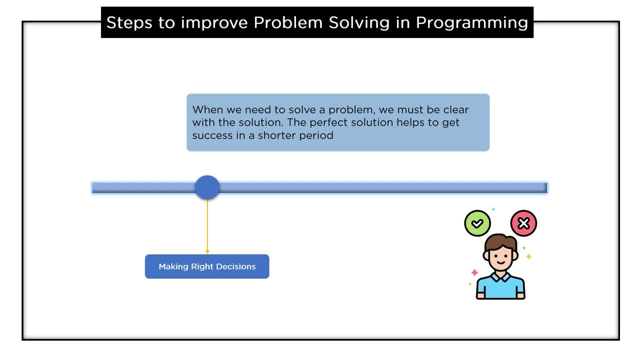 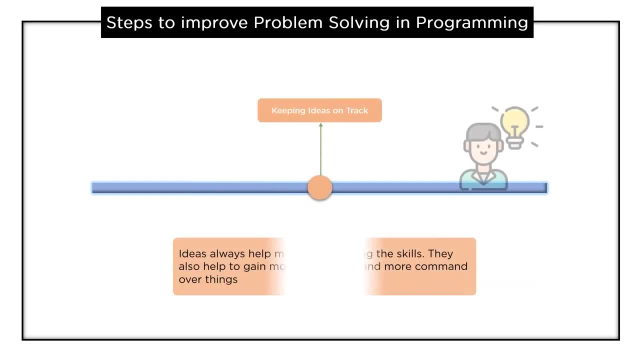 and efficiently. These skills also help to get more command over the subject. Followed by that, we have the next step, that is, keeping ideas on track. Ideas always help much in improving the skills. They also help to gain more knowledge and more command over things. 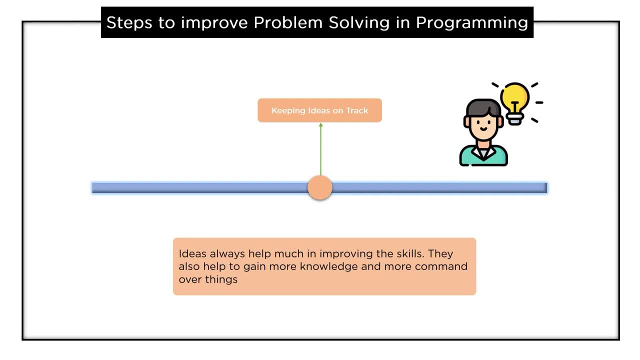 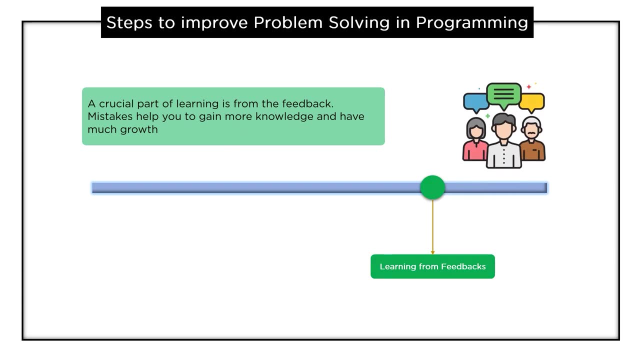 In problem solving situations. these ideas help much and help to develop more skills, give opportunities for the mind And keep on noting the ideas. Next, we have learning from feedbacks. A crucial part of learning is the feedback. Mistakes help you gain more knowledge and have much growth. 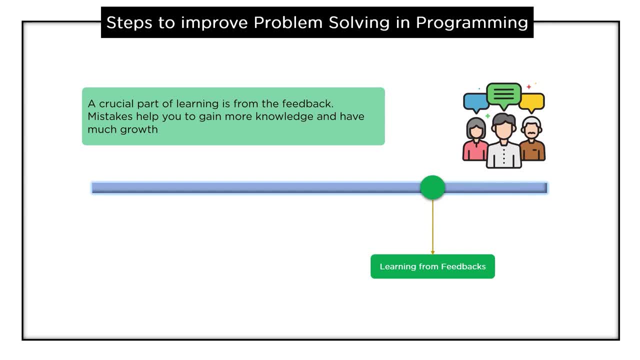 When you have a solution for a problem, go for a feedback from experienced or the professionals who are seniors to you. The last one is asking questions. Questions are incredible part of life. While searching for solutions, there are a lot of questions that arise in our minds. 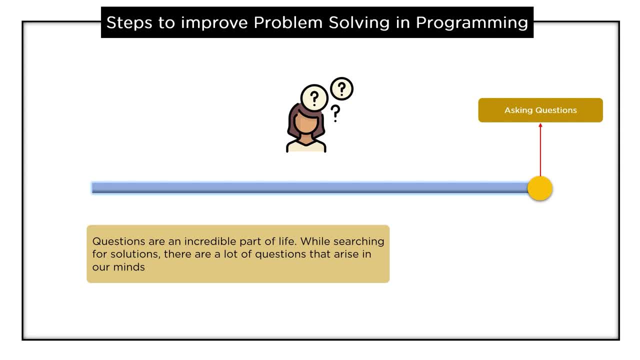 Once you know the question correctly, Then you can find answers quickly. In coding or programming we must have a clear idea about the problem, Then you can find the perfect solution for it. So these were some of the important steps to improve problem solving skills in programming. 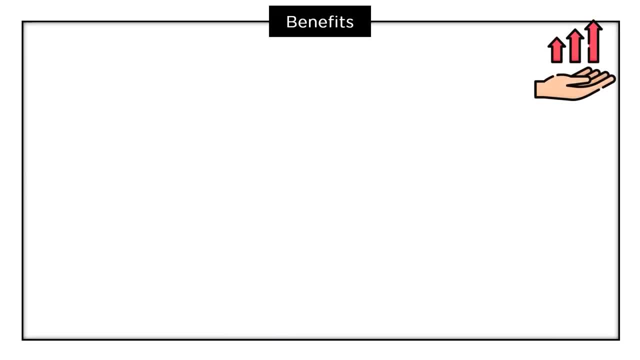 Now let's learn about some important benefits of problem solving and programming. So the first one is: the major benefit of problem solving is to gain more knowledge over coding and programming. These problem solving techniques and skills also improve the knowledge in a person. So the first one is: the major benefit of problem solving is to gain more knowledge over coding. 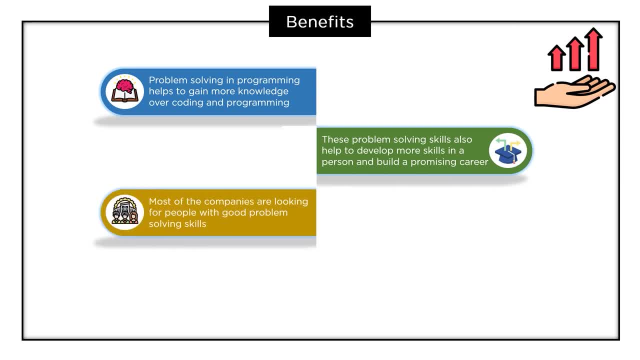 and programming. These skills also improve the knowledge in a person and build a promising career. These skills play an important role when it comes to jobs. Most of the companies are looking for people with good problem solving skills, and these play an important role when it comes to job opportunities. 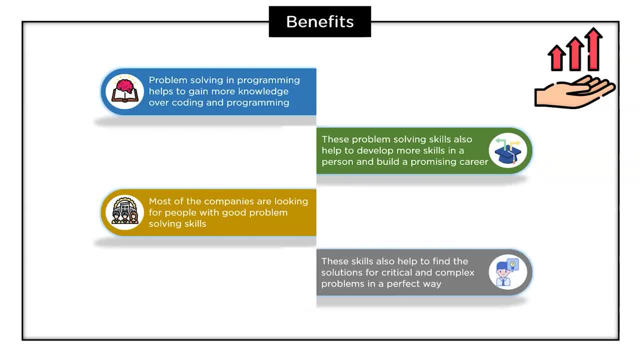 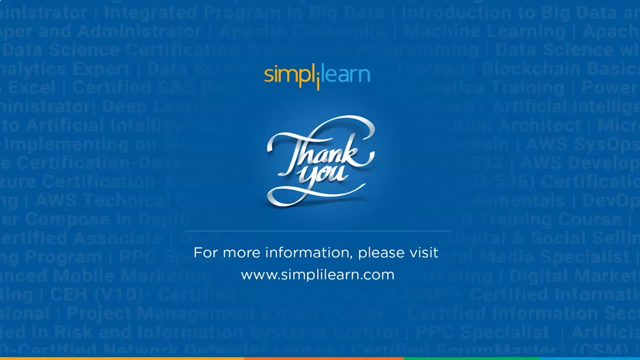 These skills also help to find the solutions for critical and complex problems in a perfect way. And this was all for today's session. I hope now you guys have got an idea of how important problem solving is in these days. If you find the information helpful to build a good job, please share it with your friends.